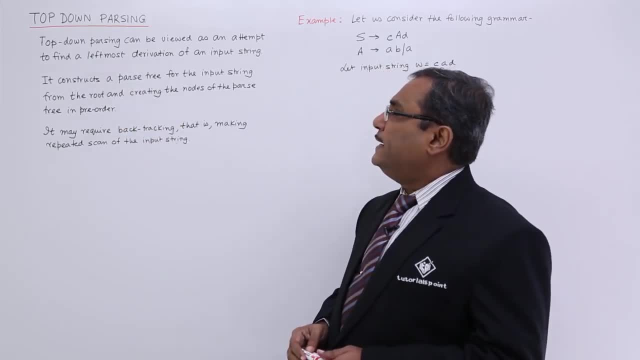 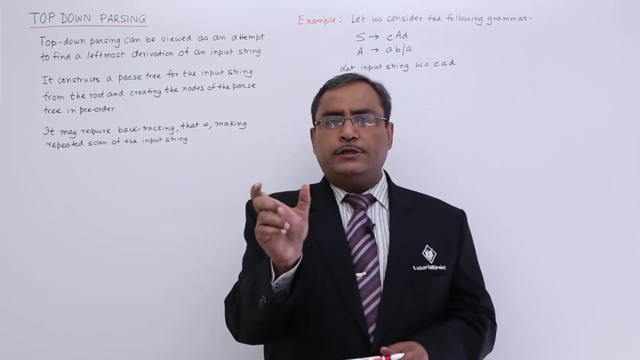 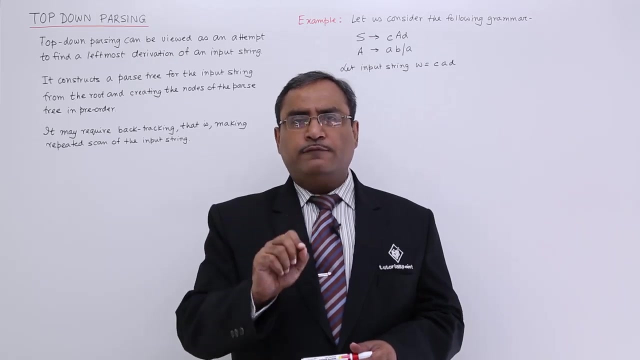 See top down. parsing can be viewed as an attempt to find the left most derivation of an input string. We know that in the sentential form it will be a collection of terminals and non-terminals, And left most derivation means starting from the left hand side. the first non-terminal will 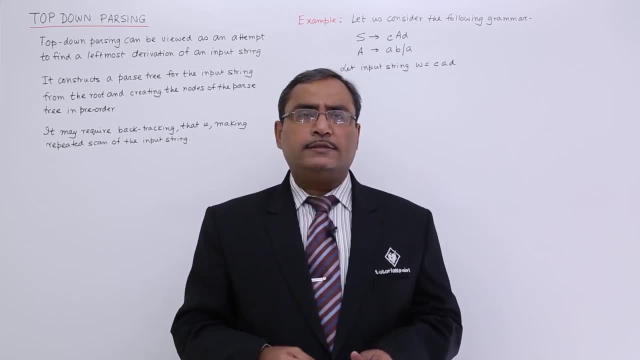 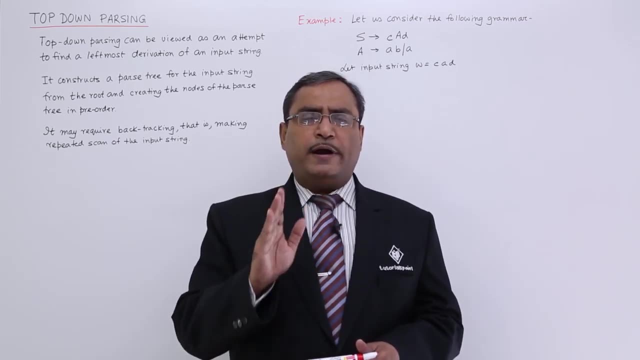 be replaced with the respective production rules: right hand side, So that is known as the left most derivation. So that means at first from the left hand side we shall find out the handle, and the handle will be replaced by the respective handle production, So that 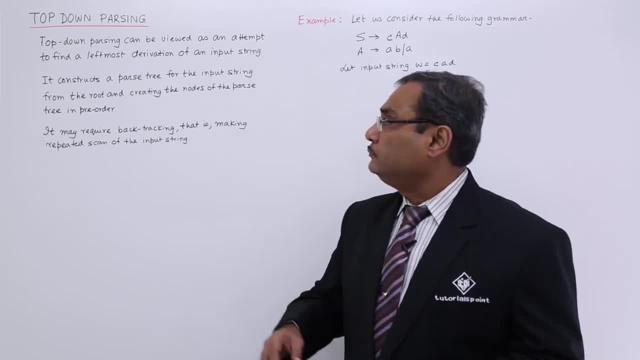 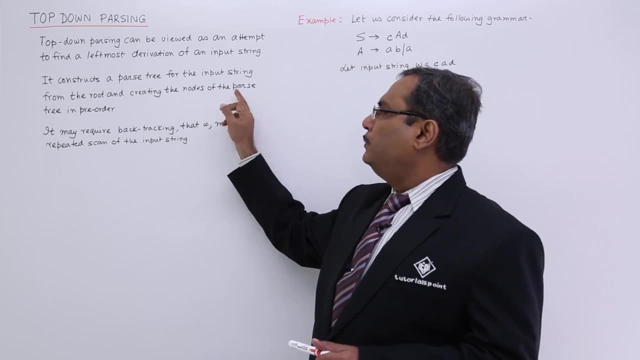 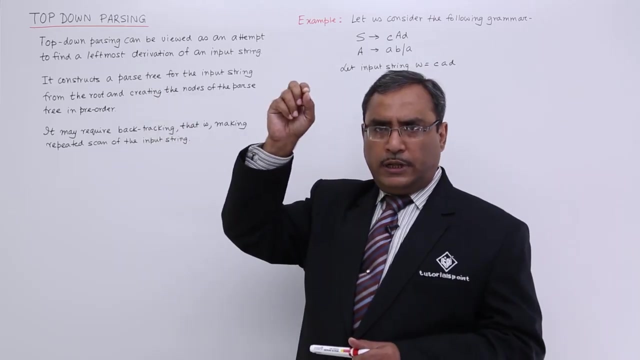 is the left most derivation Now see it constructs a parse tree for the input string from the root and creating the nodes of the parse tree in the preorder. So what is the meaning of this? it will start parsing from the root node. that means it is. 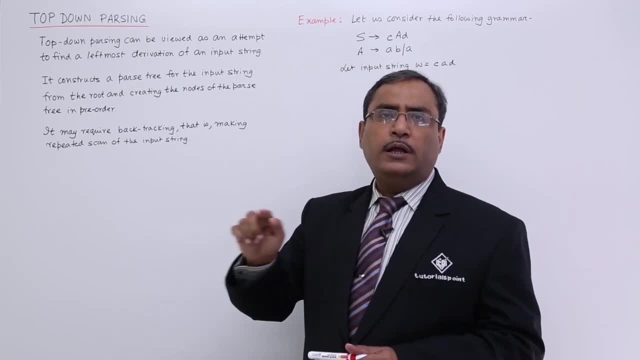 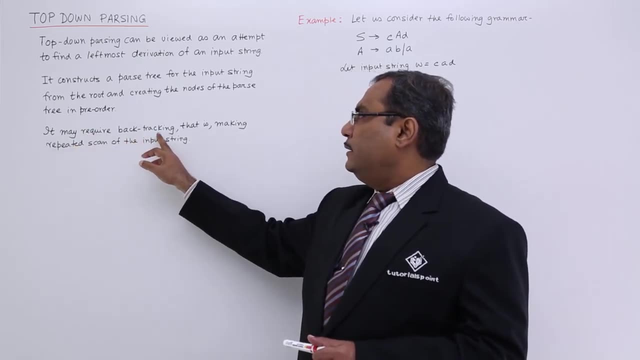 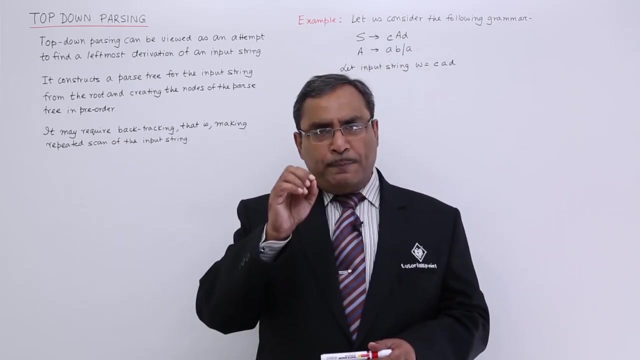 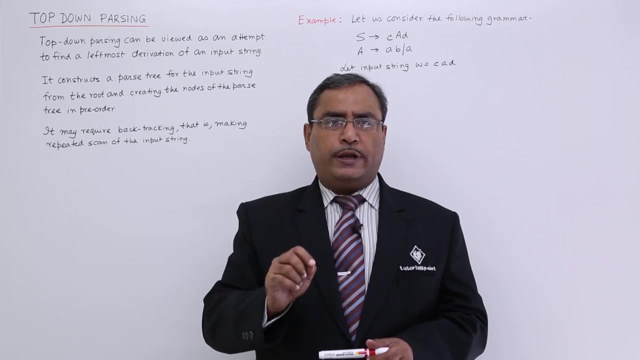 top down it will come from the root node and then it will go to the leaves leaf nodes. that means the input string. It may require backtracking, that is, making repeated scan of the input string. So sometimes it may happen that from a particular non-terminal we are having multiple production rules to to get the respective input string. 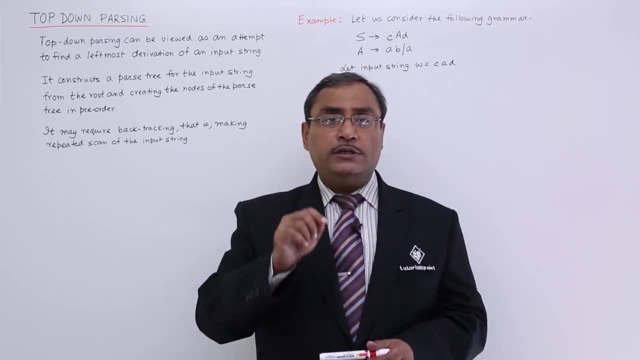 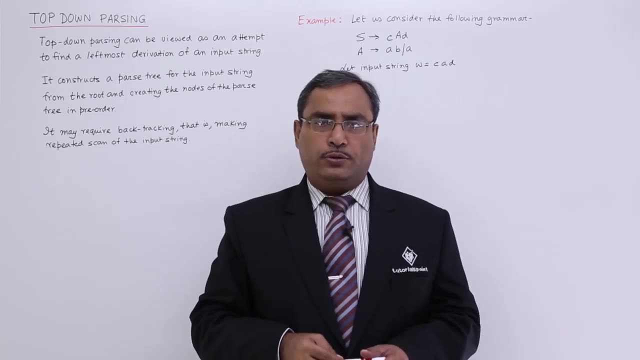 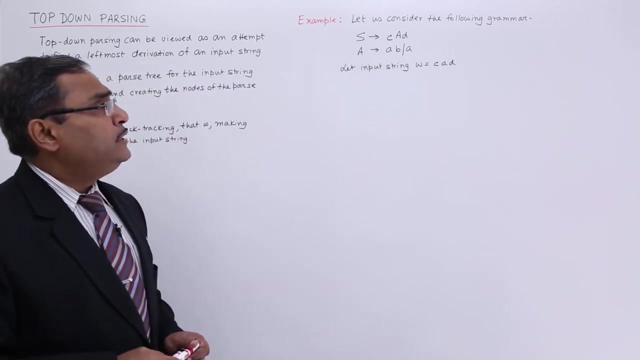 we might have used one of them, but that is not generating the input string later on. then we may backtrack and then you shall apply with the new production rule. So if the things are not clear to you, let me go for an example. So let us suppose that 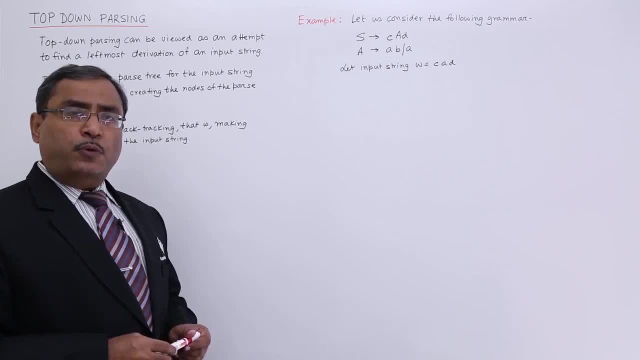 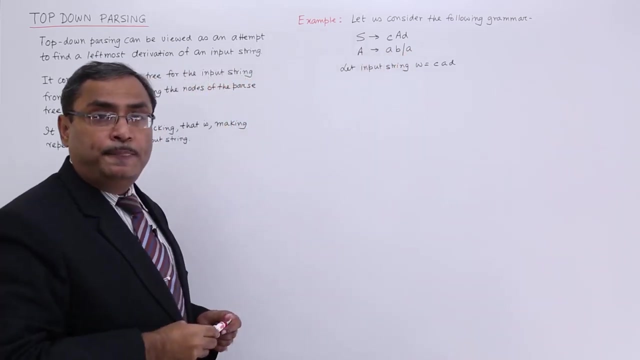 is one grammar is given: capital S produces small c, capital A small c, capital X and capital small d and capital A produces small a, small b and small c small a. So that is or is this one. So A produces a b and A produces small a. So two production rules are there. 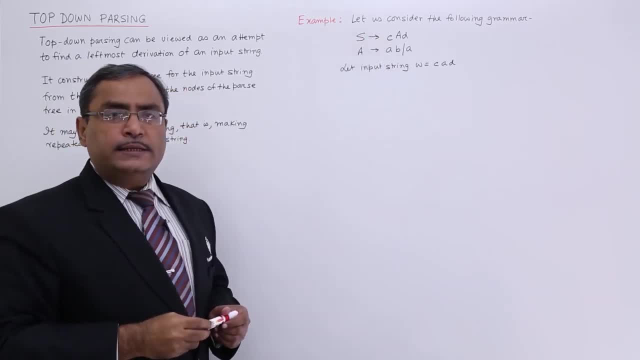 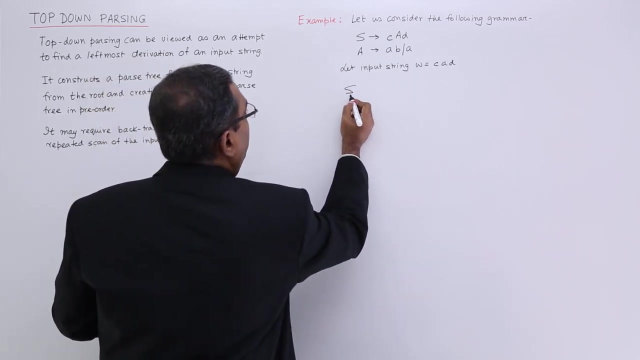 here. and one production rule is there: Let input string be c a d. The input string here is c a d, So let me proceed. So here I will be using the top down parsing. That means I will be starting from the start symbol s Now. at first I shall go for s produces c. 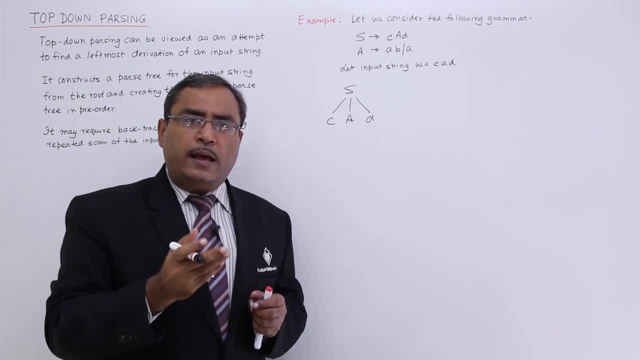 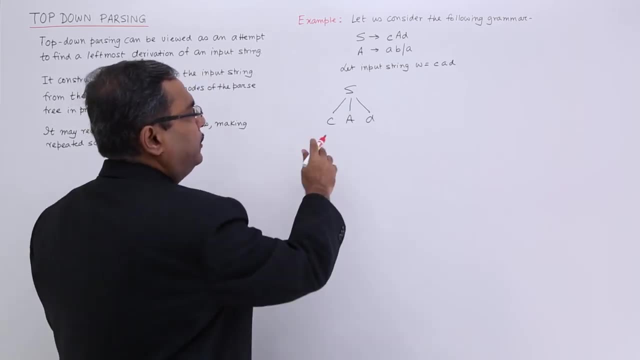 a d, because there is no other way, because from the start symbol we are having a single production rule that is c a d. So now just scan the input and this particular yield. So here we are having small c, here we are having small c. So we are highly optimistic. 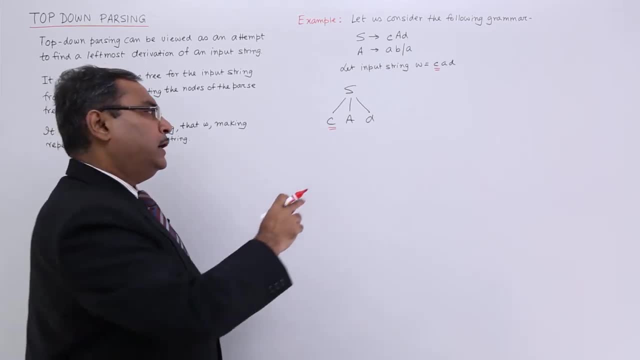 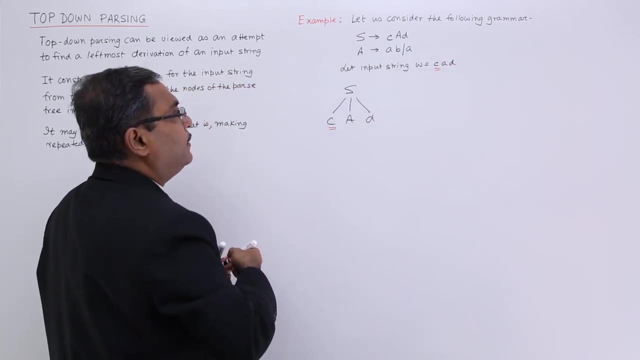 that we are going to get the input string, So, but the next one is capital A. but here I require a small a. So let me go for this: production a, b. So A produces a, b, So I am applying this one. So now, here you see, this small. 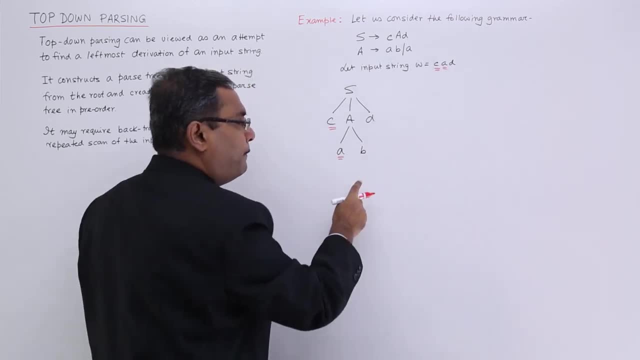 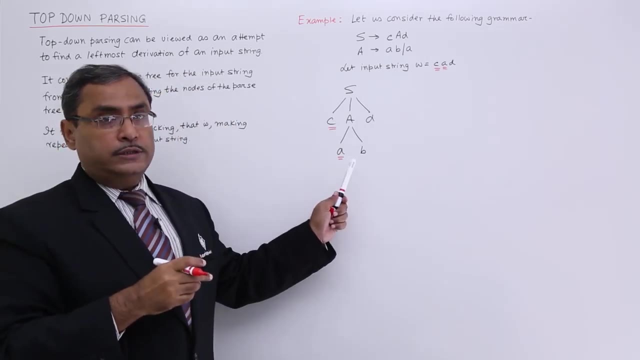 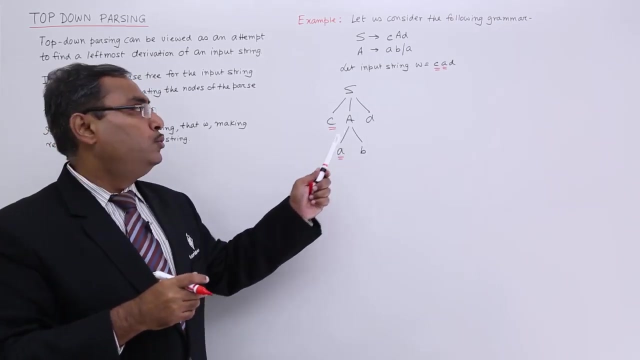 a is also corresponding to this small a, but here I am getting b, but that has no b here. That means this production rule is not correct. I should try with the other production rules. So I shall do the backtracking. That means I shall do undo here. So I will be getting. 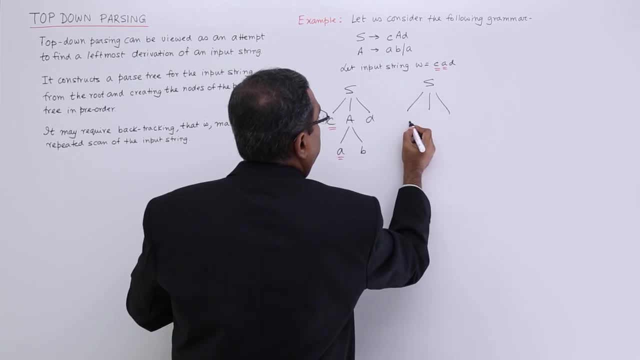 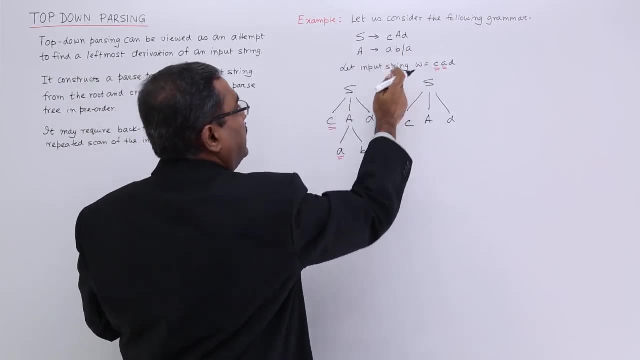 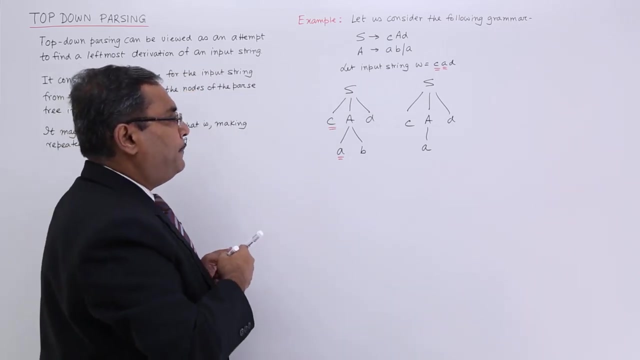 that s produces c a d back. I shall go for the backtracking Now. I shall apply the other option, that is, small a. So I shall apply small a here After doing the backtracking. I am applying small a. So what will happen? So c we matched earlier, So here we are. 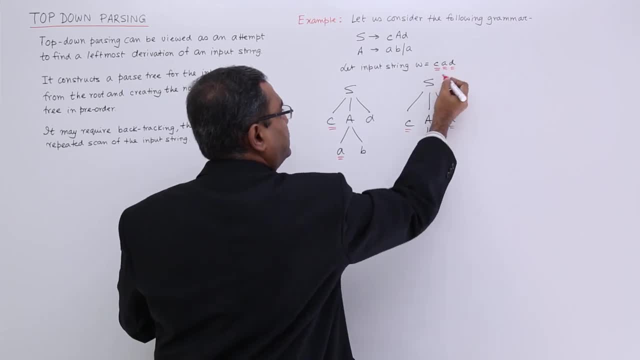 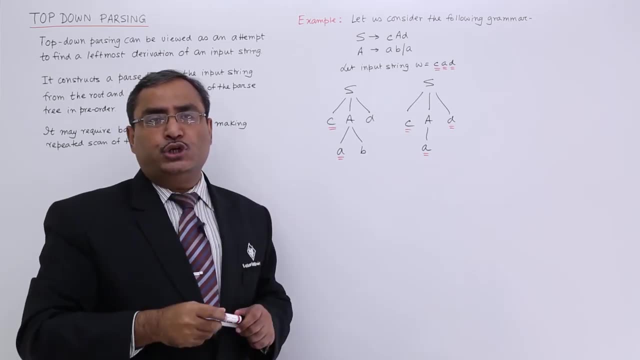 having a, it is matching. and the next I am getting d, also it is matching. So I got my input string that is c a d. So here the parsing will tell that successful completion of the parsing and this particular c a d is ok and we are accepting this one, This input string. 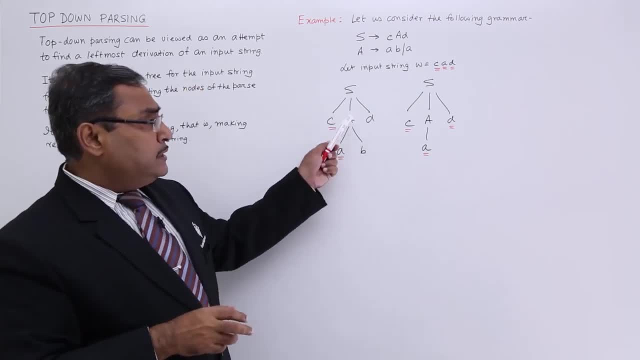 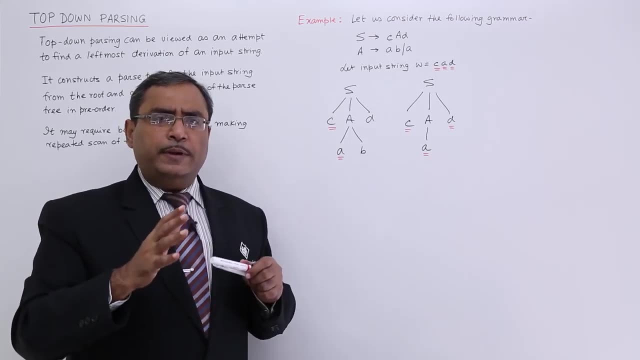 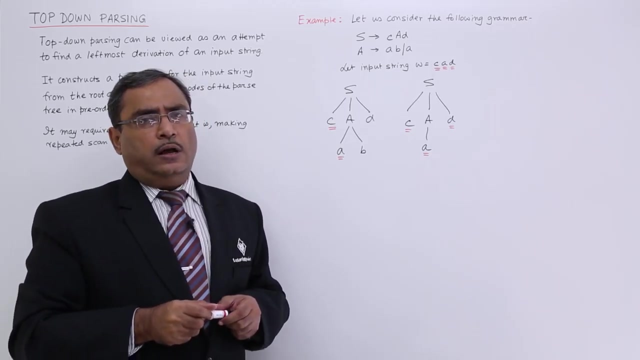 is getting accepted by this parser. So this is the main disadvantage, that is, the backtracking. To resolve this backtracking, obviously you must be having some method, Otherwise top-down parsing will not be applicable. So we are having recursive descent parser and where 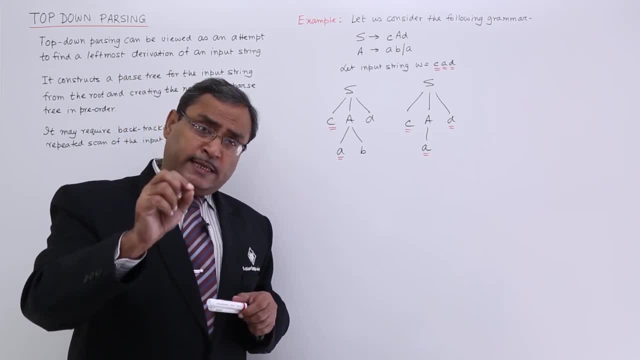 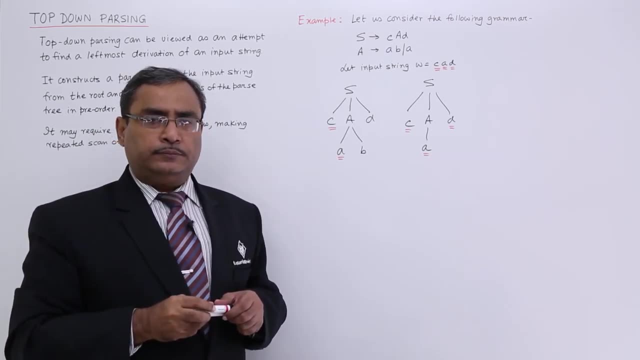 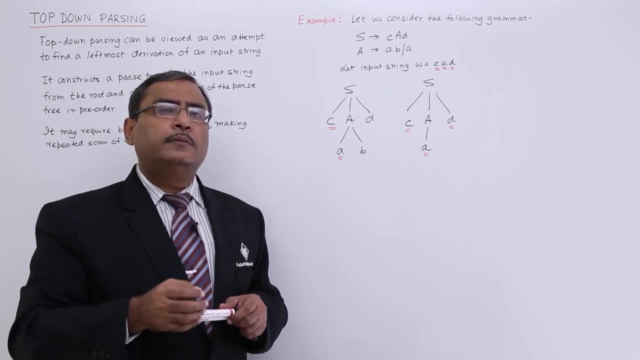 we will be having our predictive parser, where the parser itself will tell that, to get this particular input string, what production we are supposed to apply. Regarding this predictive parser and all, we are having a separate video in the next topics. You can easily watch them: how we can construct the predictive parser, how we 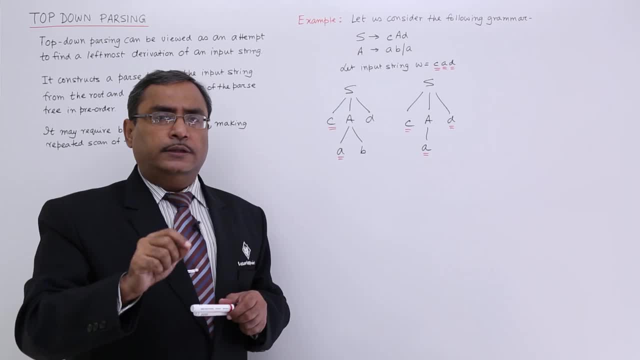 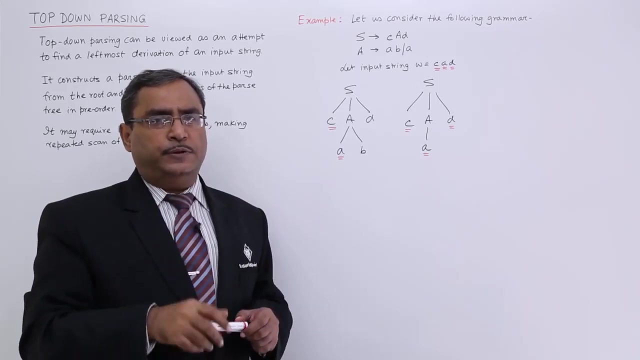 can construct the recursive descent parser, how we can construct the recursive descent parser So that this sort of backtracking can be avoided and parser will have a parsing table and from the parsing table we shall get a clear-cut idea that which production rule has to be applied to get the input string parsed successfully, If it can be parsed successfully. 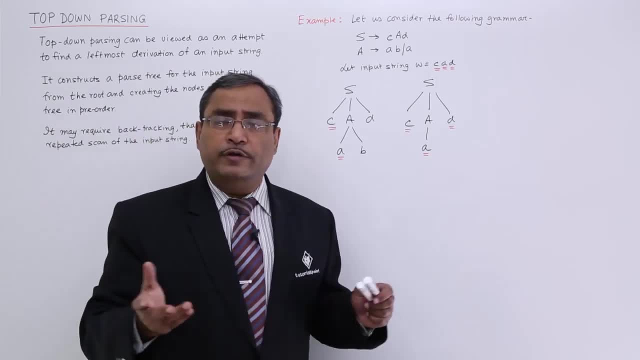 obviously, but if it is not in accordance with the production rule, obviously that case also it will produce error messages. So everything will be discussed in our next videos, but for the time being this is my presentation. Thank you very much. 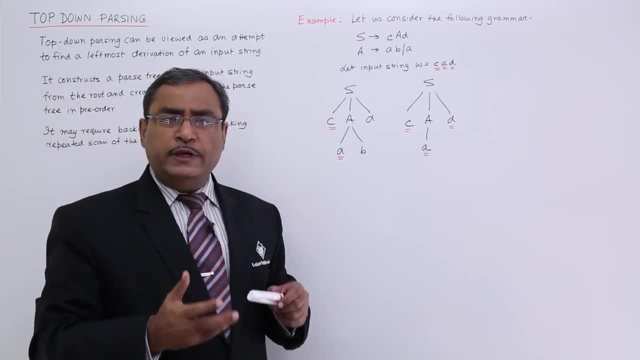 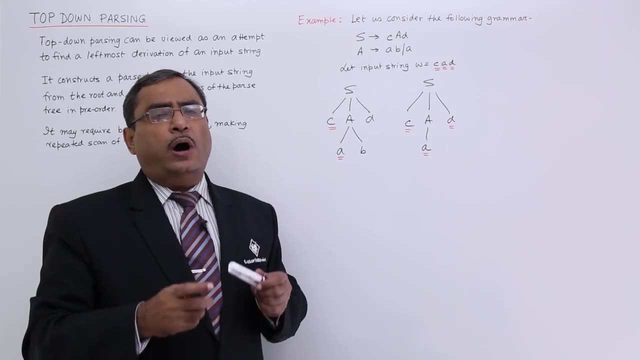 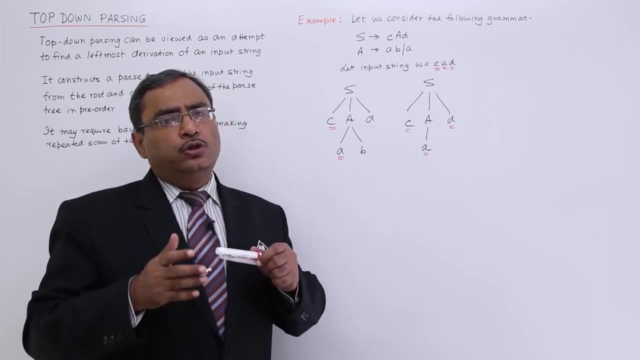 1. How to write production rules. I have written, but obviously this production rules cannot be taken by the parser directly, It must be written in some code. So how to write code, program code against the production rules, How the production rules can get expressed. 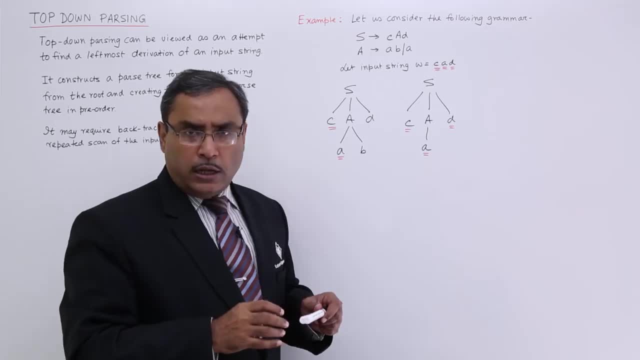 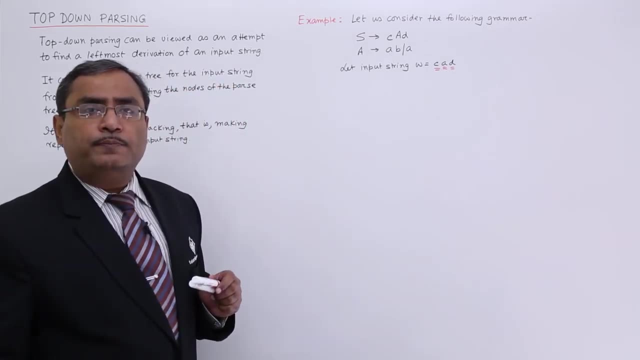 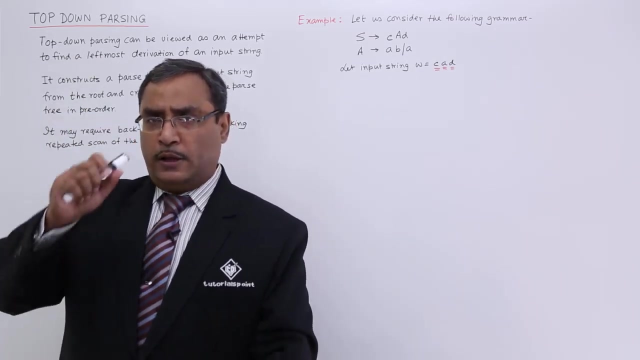 through programming code. I shall explain that one here. Please let me allow to write the respective code against this particular production rule. So for the first one we are having: S produces C, A, D. So I am writing the respective program code against this particular. 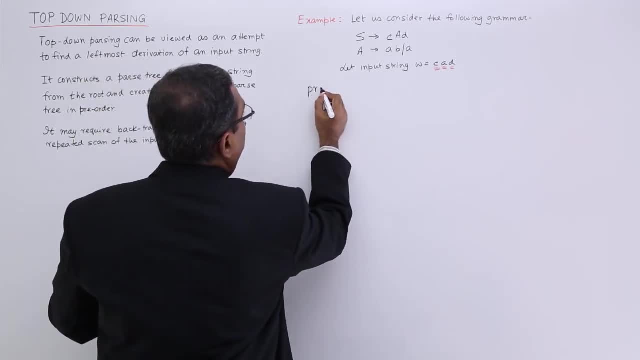 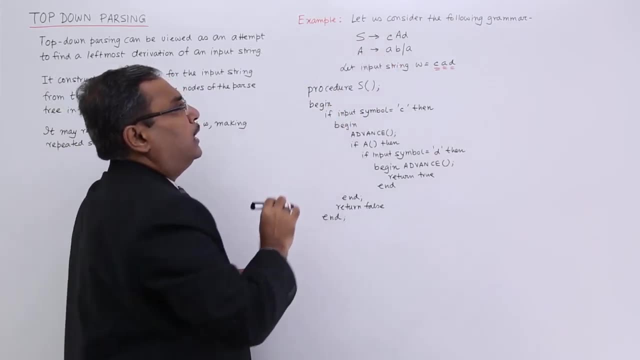 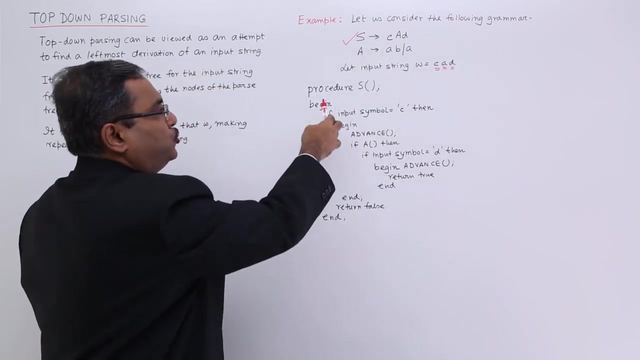 production rule 2. Now I have written this particular program segment for this first production rule. It is for S produces C, A, D, 5. So procedure S. So this S is corresponding, this one. if import symbol is equal to small C, So it is for S produces C, A, D or for entire points, all S will be equal to small. 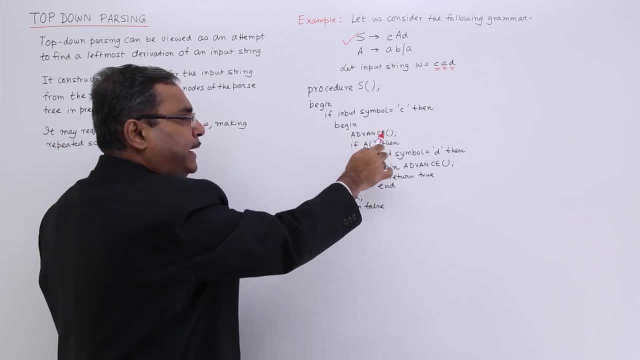 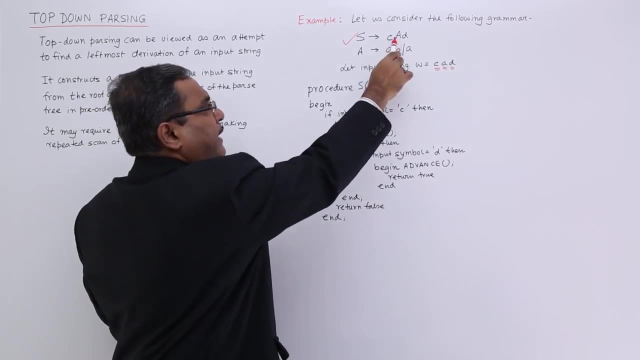 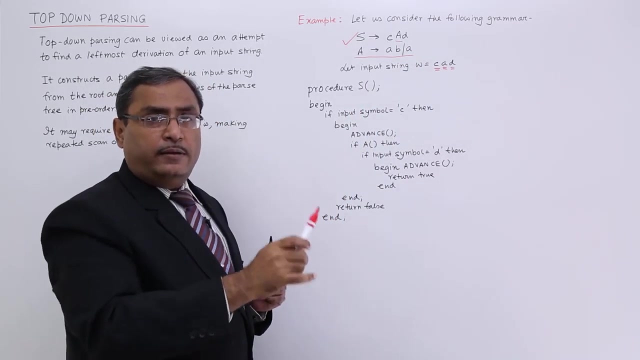 the first one, i am writing this one, then begin advance, then i shall go for the next string, next symbol to be read: if a, because a is a non terminal and it is having a separate production rules, so i shall have to write another a i shall be writing another that particular procedure. 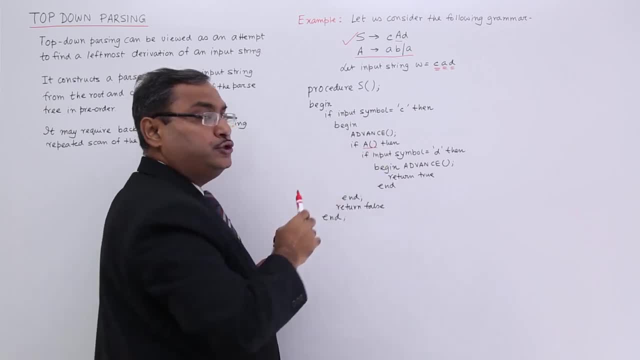 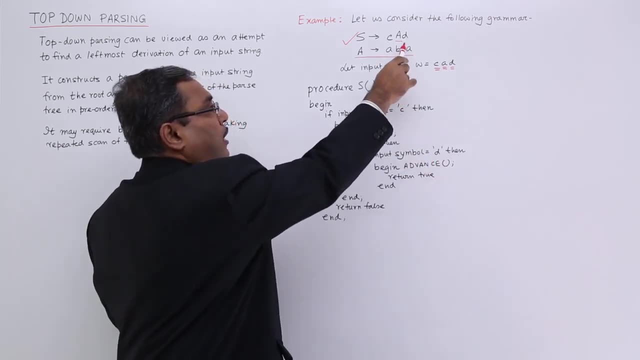 a will be called here. so that is why i have called this particular procedure a. so procedure a has to be written separately. then if input symbol is d. so now if the input symbol is d, then begin advance return. true, that means my c a, d have got recognized. so from here. 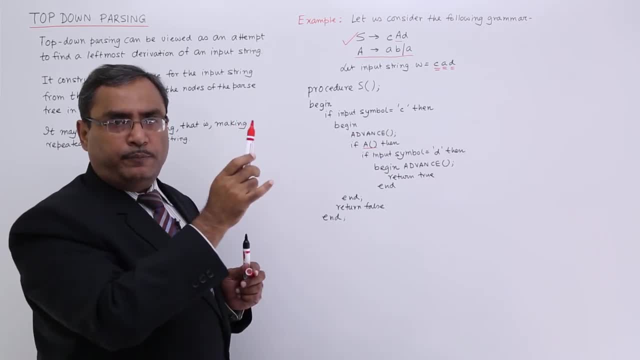 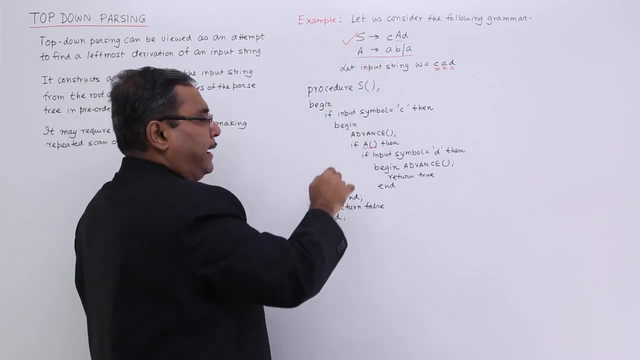 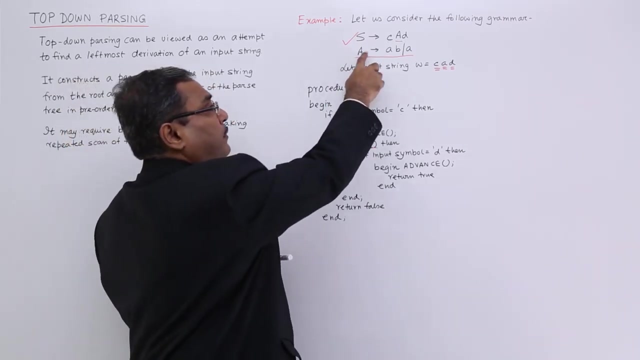 i shall terminate. i shall return to the caller from where the my program has been called end. otherwise i shall return false and end in this way. the same. this production rule can have the respective program code. so let me write the procedure a to have the completion of this. ok, i have completed this. 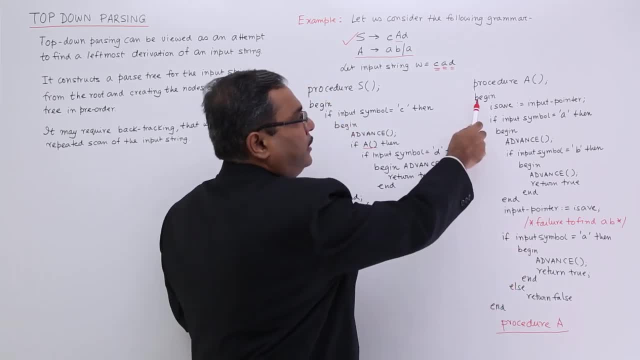 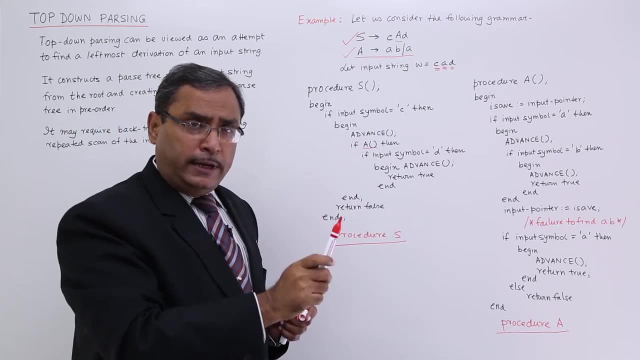 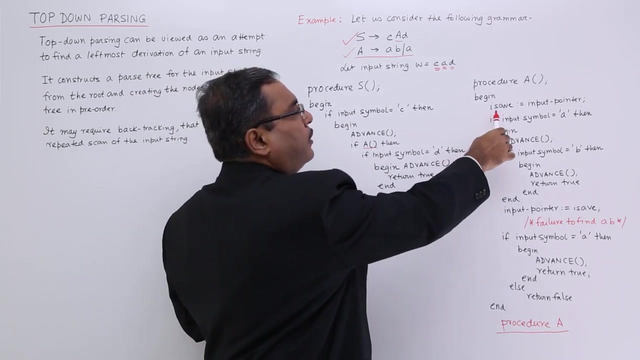 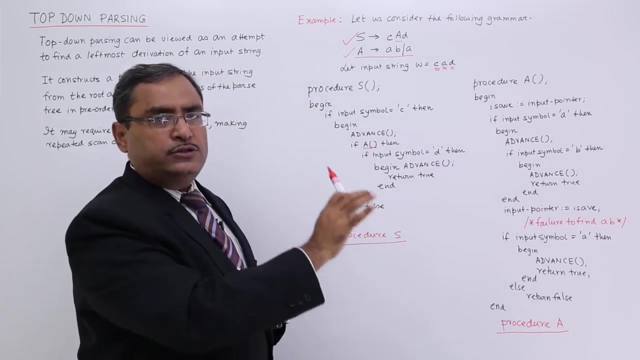 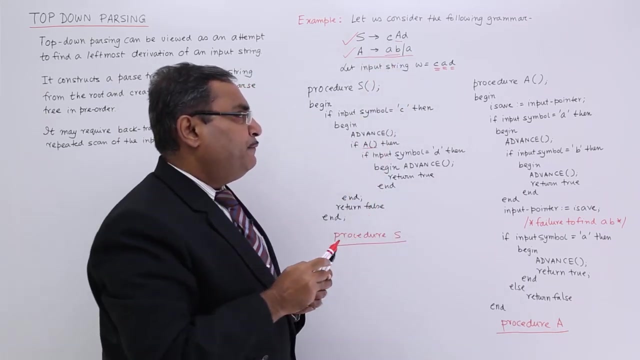 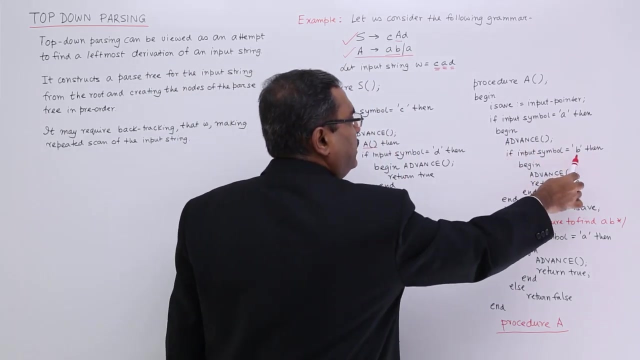 particular procedure a c, procedure a: that means i am writing the code for this production rule. here we are having two production rules: capital a produces small a, small b, and capital a produces small a. so this block moment, and i shall do it, that means i shall say that the result of this c? u a is d? B. this will be: 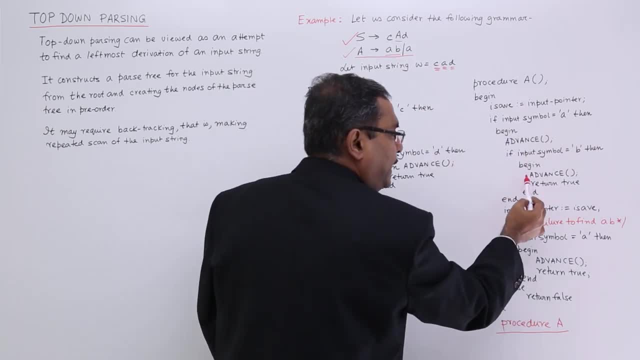 done by this: if this c? u a is d, by two of the same way. that is why i have red. so important things here, which i will do first. start with b in small b, until i finally turn theseices: yes, this c? u a is D, as well as c? u a dash left and d dash k. let me in by this b, D, a, and then 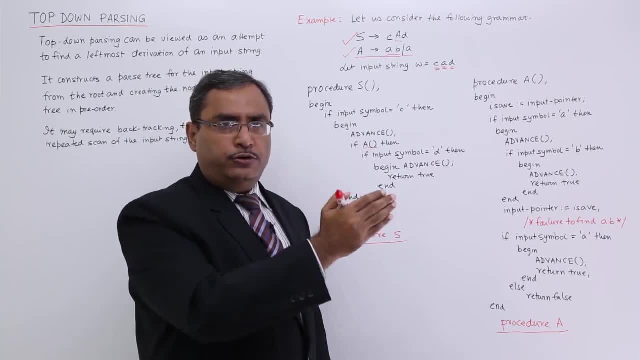 then return 이것도 a to add it, just like i say we. that meansNo structure. so we have an barrier which go for six p a day. it allows us to add all the chap ups. united ec question. true, because i got a and b so i should return true end. so that is the ok. but if it is not, 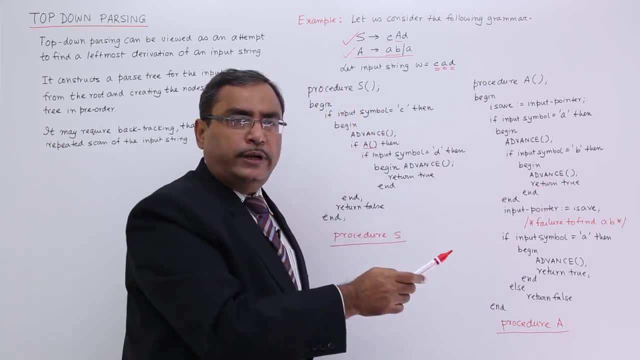 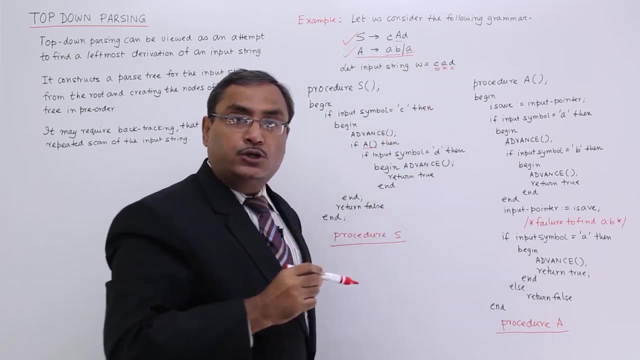 getting terminated. that means if the return true is not getting executed, then contour will be coming to the next line. that means a, b has not been obtained. so i should go for a checking now. i should go for a checking. so in this case it is doing if input symbol. 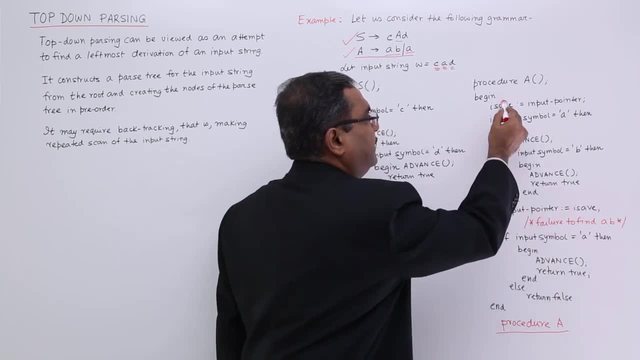 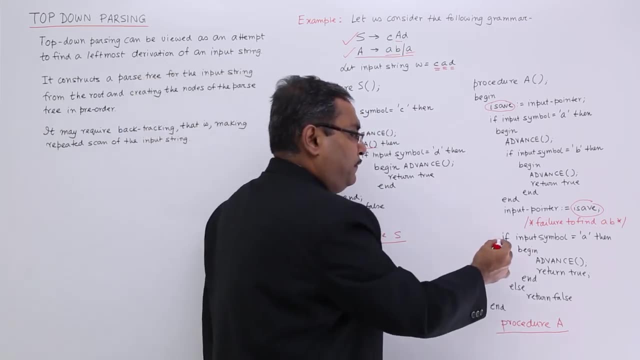 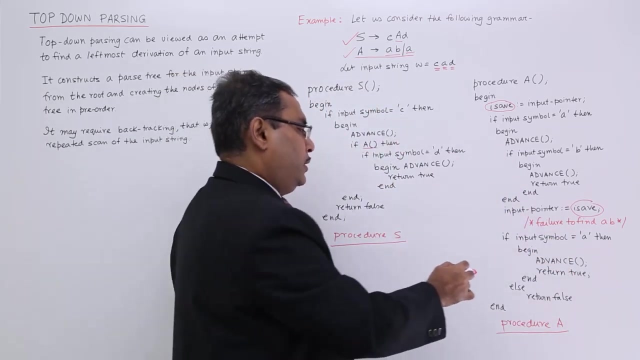 so now input pointer is now getting initialized with this. i say: whatever i kept, value is now getting assigned to input pointer, so i am retracking. so if input symbol is equal to small a, then advance return true. that means i got a, so i should return true, else return. 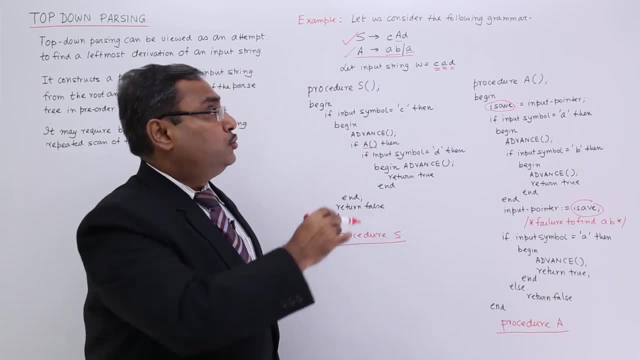 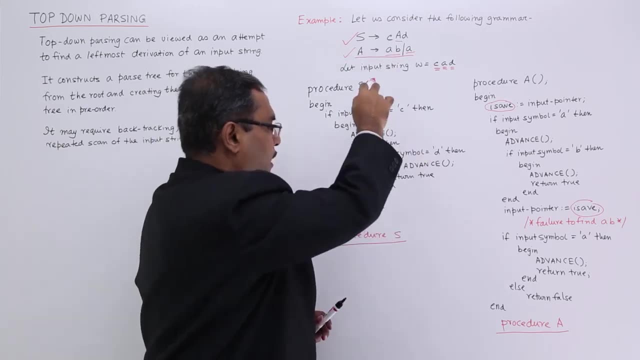 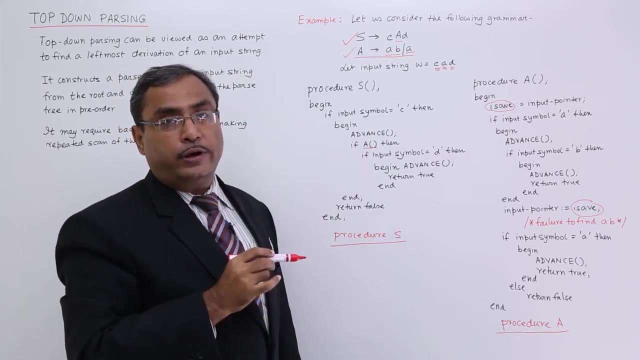 false and this begin is having this end. so this is my program ah segment written against this particular production rules. so this is my production rules and these are the program segments. how to write the program segments against the production rule. we have shown that one very elaborately.